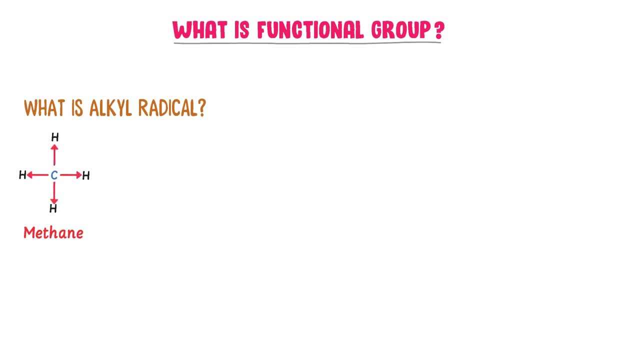 In this molecule of methane, carbon forms four single bonds with four hydrogen atoms. Now if I remove this one hydrogen atom from this methane, then it becomes alkyl radical. So this is alkane molecule and this is alkyl radical. It is represented by capital R dash. 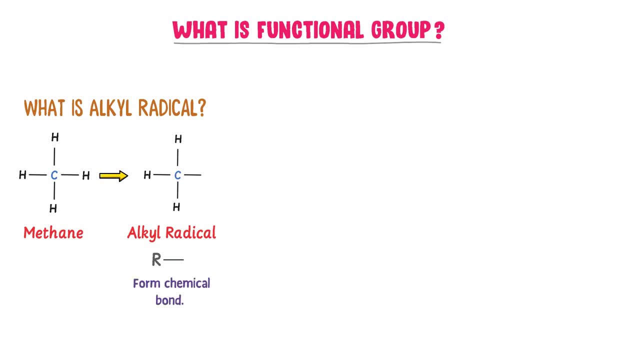 This dash means that it can form chemical bond with other species. Now I take this alkyl radical, I attach OH to this alkyl radical And I get something new. I mean, I get alcohol. So OH changes the function of alkyl radical. 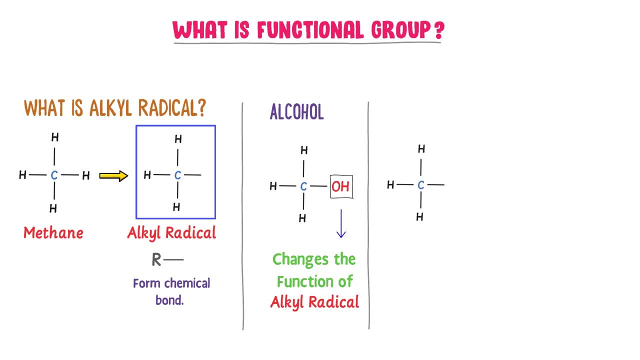 Secondly, I take this alkyl radical. This time I attach COOH to this alkyl radical And I again get something new. I mean, I get carboxylic acid. So COOH changes the function of alkyl radical. 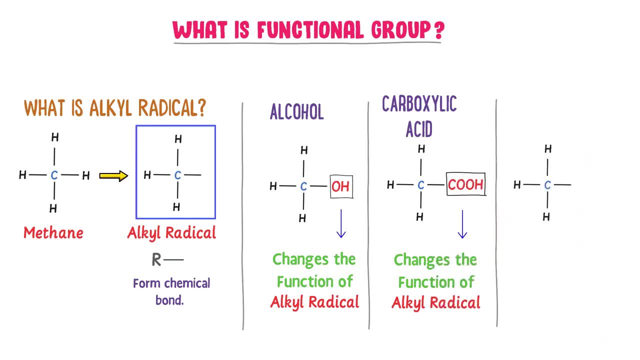 Thirdly, I take this alkyl radical. This time I attach CHO to this alkyl radical And I again get something new. I mean, I get aldehyde. So CHO changes the function of alkyl radical. Now listen carefully. 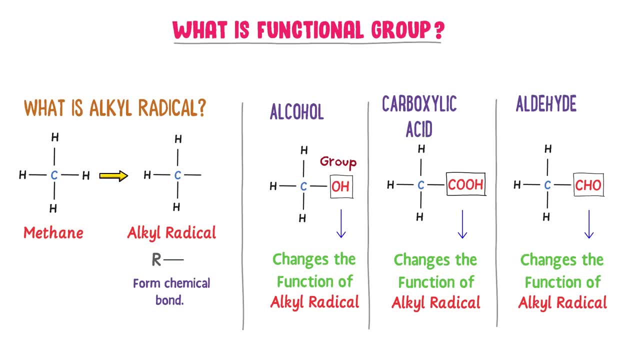 This OH group of hydrogen and oxygen atoms change the function of alkyl radical and make it alcohol, So we say that it is a functional group. Secondly, this COOH group of carbon, oxygen and hydrogen atoms change the function of alkyl radical and make it carboxylic acid. 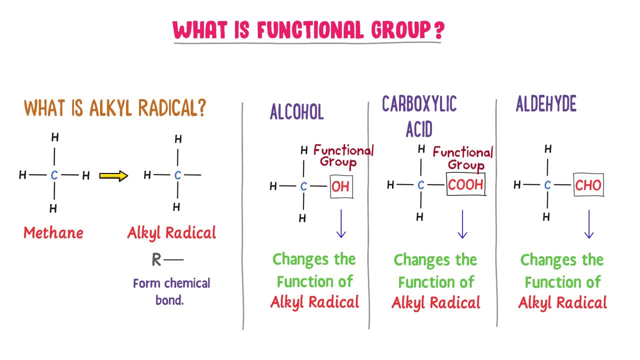 So we say that it is a functional group. So we say that it is a functional group. Thirdly, this CHO group of carbon hydrogen and oxygen atoms change the function of this alkyl group and make it aldehyde. So we say that it is a functional group. 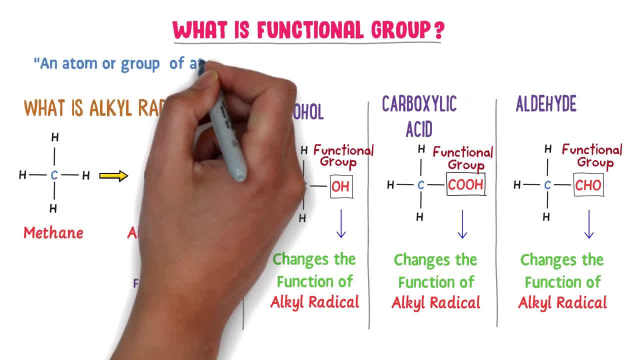 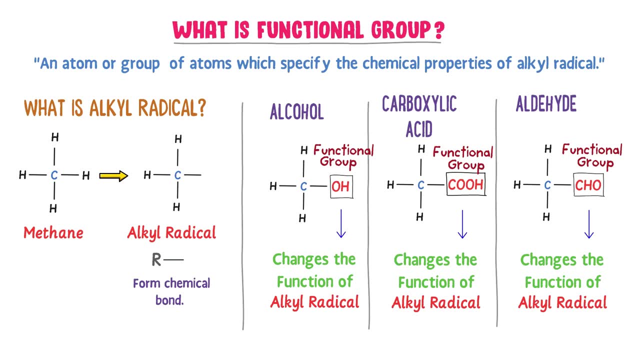 Thus we define functional group as an atom or group of atoms which specify the chemical properties of alkyl radical is called functional group. Let me repeat it: An atom or group of atoms which specify the chemical properties of alkyl radical is called functional group. 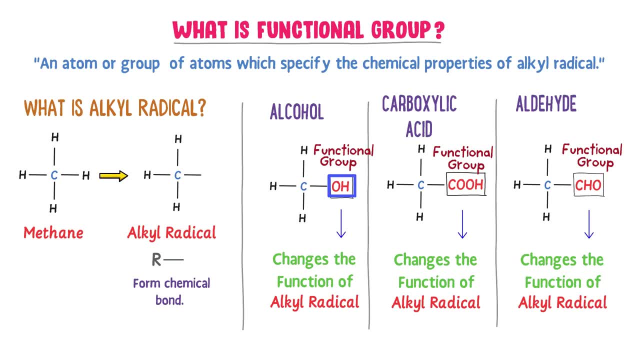 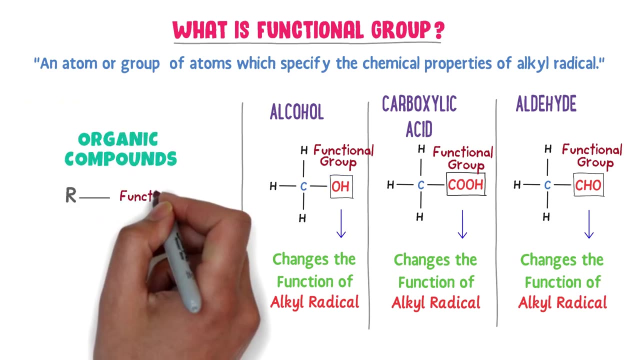 For example, OH is a functional group that specify the chemical property of this alkyl radical, And without this OH group it is a simple alkyl radical. It is no more alcohol. Thus, the general form of any organic compound is R-functional group. 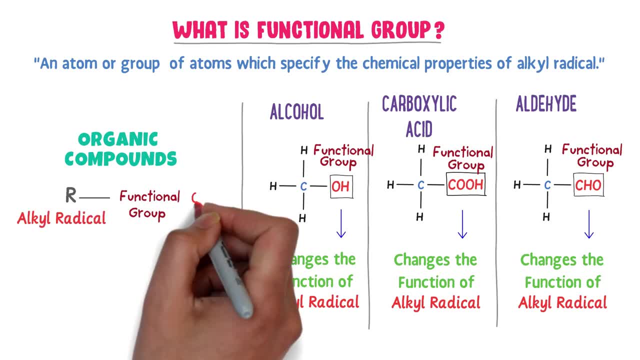 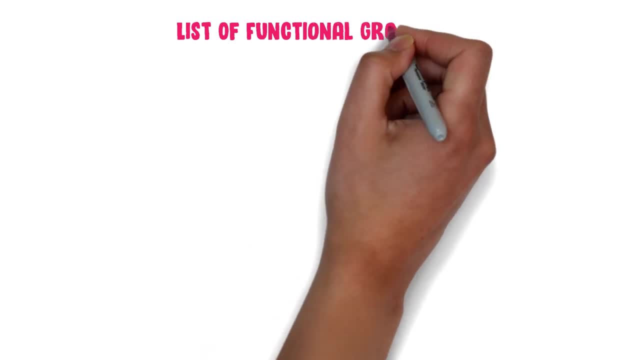 where R is the alkyl radical and we can attach different functional groups to this chemical group. So we say that it is a functional group to this alkyl radical. Now let me teach you the list of important functional groups. Firstly, I always write. 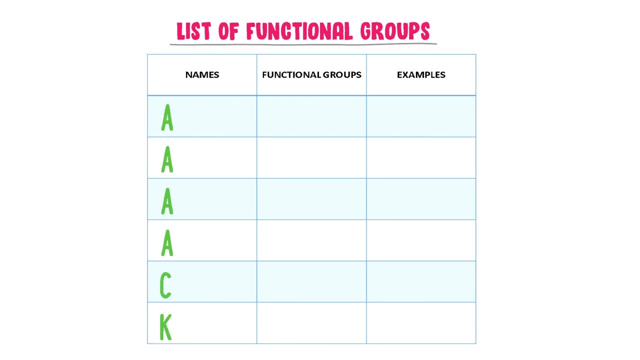 4S, C and K. 4S stands for alcohols, aldehydes, alkyl halides and amines, C stands for carboxylic acids and K stands for ketones. The functional group of alcohol is: 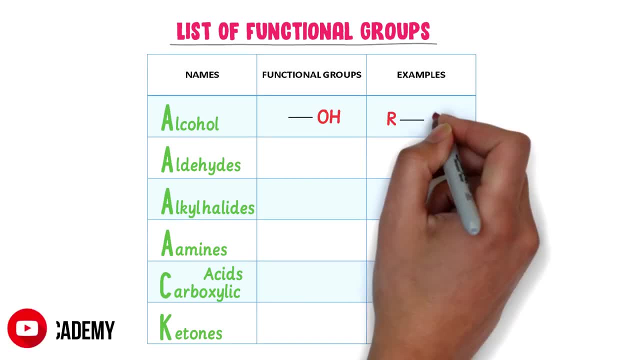 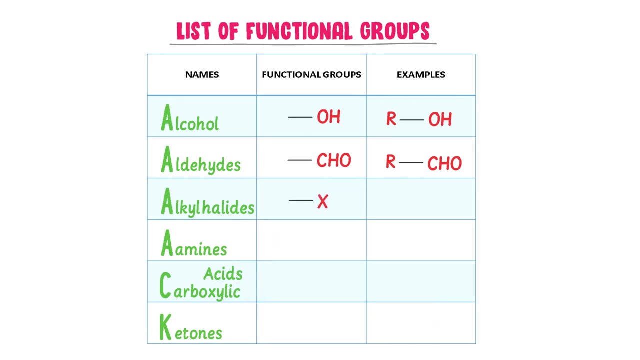 dash OH, For example R-OH. The functional group of aldehydes is dash CHO, For example R-CHO. The functional group of alkyl halide is dash X. This X represents halogens like fluorine, chlorine, bromine, etc. 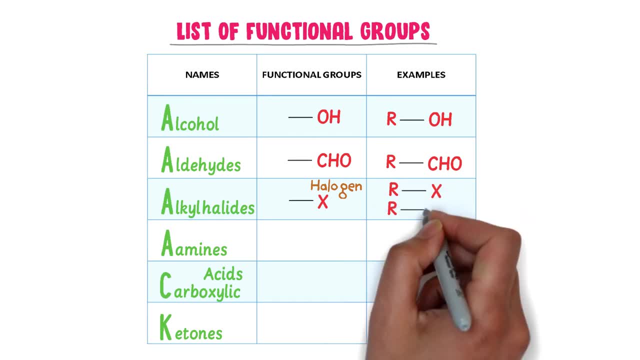 For example R-X or R-BR. The functional group of amines is dash NH2.. For example, R-NH2.. The functional group of carboxylic acids dash CHOH, For example R-CHOH. 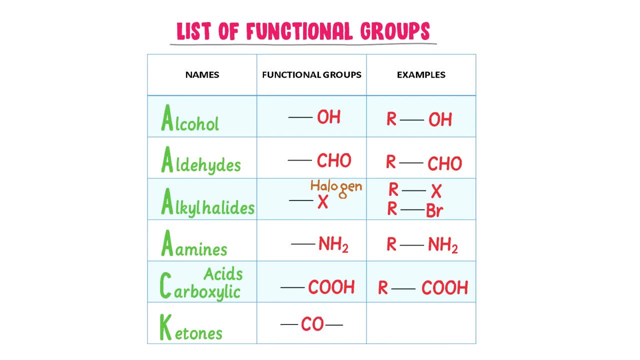 And the functional group of ketones is dash CO', For example, R-CO-R. This is the list of all important functional groups which we study in organic chemistry. Just note it down, this list of all important functional groups. Finally, let me teach you the method of. 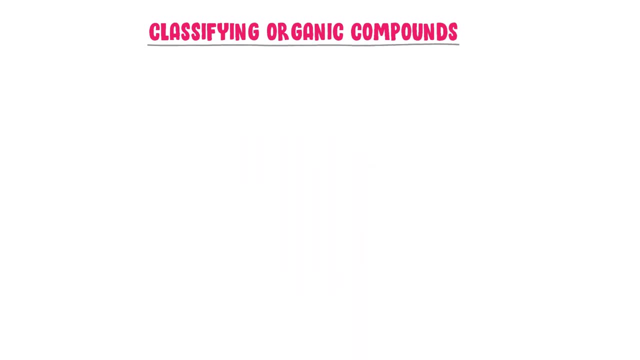 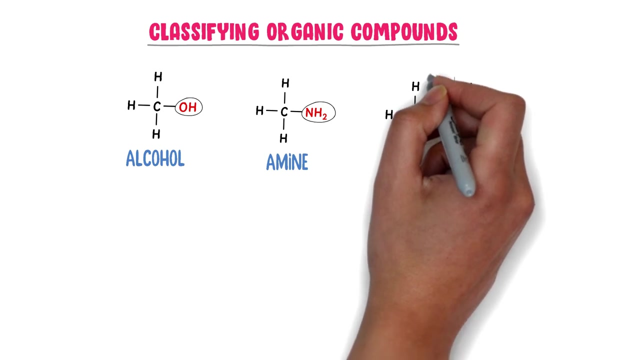 classifying organic compounds on the basis of functional groups. For example, this is alcohol because it contains OH group. This is amine because it contains NH2 group. This is ketone because it contains CO group. This is carboxylic acid. 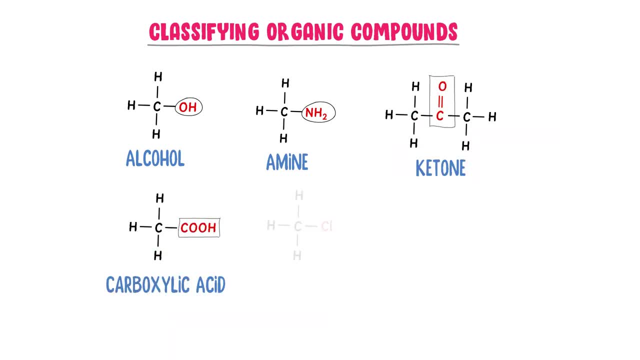 because it contains COOH group. This is alkyl halide because it contains halogen group, like chlorine. Therefore, remember that functional group is an atom like chlorine or group of atoms like COOH, which determines the chemical properties of organic compounds. 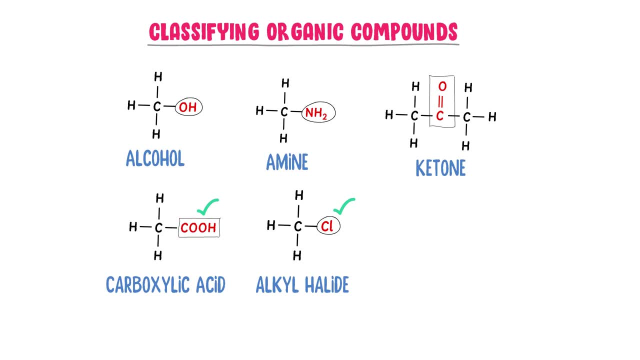 I hope that you have understood the concept of functional groups.